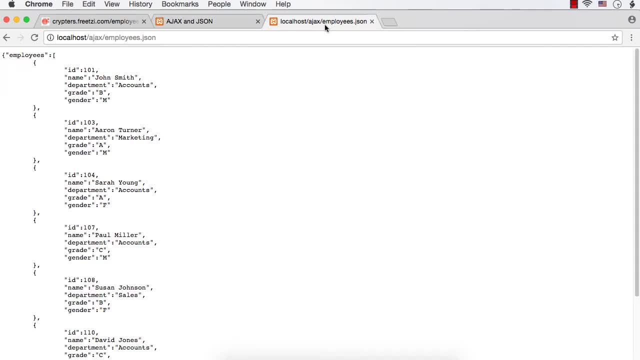 Suppose I upload this employeesjson file in an actual server Here, both this page, that is, the HTML page, and also this JSON file Both reside in the same local server folder, that is, in the ajax folder. Now suppose I access this employeesjson from a different server. 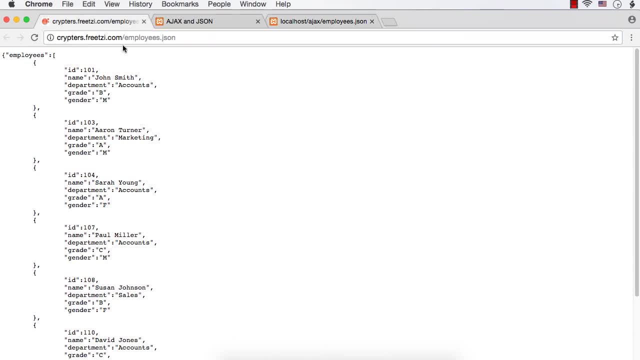 Here I have uploaded the same page that is employeesjson in a real server, which is actually a free server, And it is cryptosfreetccom slash employeesjson. So this time let me try to copy this, And here, instead of providing this, I am going to copy this: 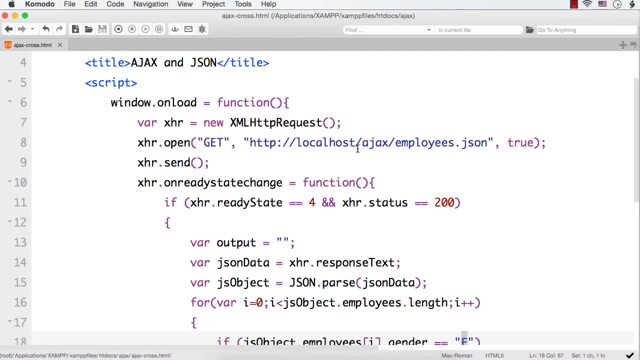 And here, instead of providing this, I am going to copy this. And here, instead of providing this, I am going to copy this. Now, I am providing this employeesjson, which is in the local server. Now, I am providing this employeesjson, which is in the local server. 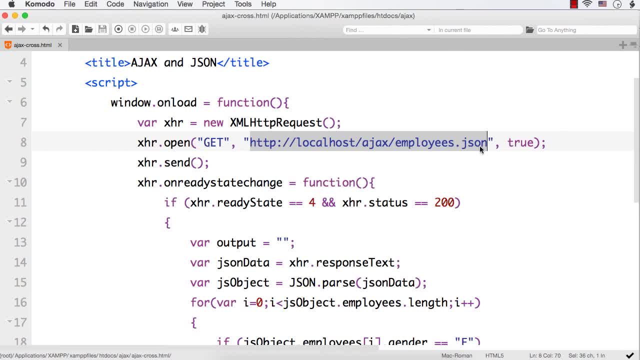 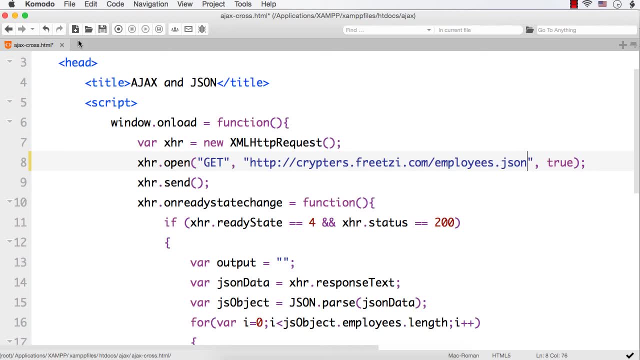 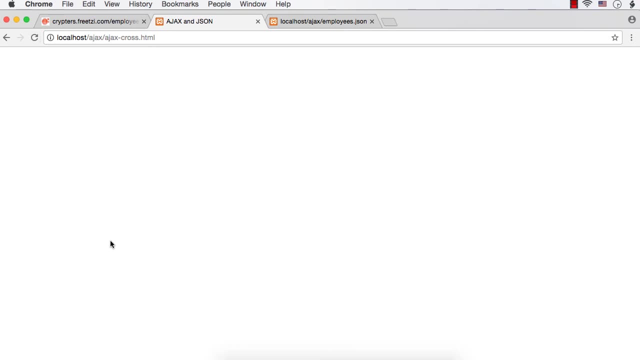 Let me put this address. Both are having the same file. okay, So it is http//cryptosfreetccom- slash- employeesjson, which is this file. Now let me try to refresh this page. See, we are not getting any output. 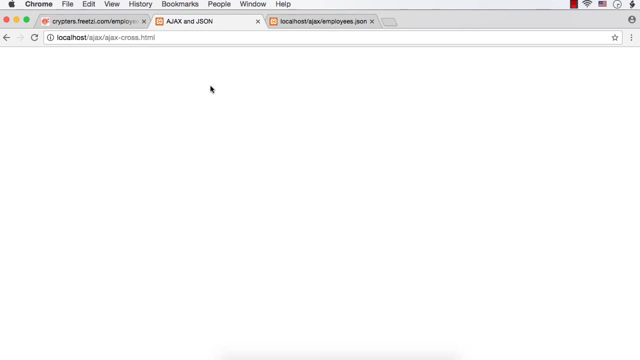 Why It is because of same-origin policy. So what is same-origin policy? So what is same-origin policy? same origin policy. scripts running in a browser are allowed to make request to only pages on the same domain, that is, the request must have the same protocol. 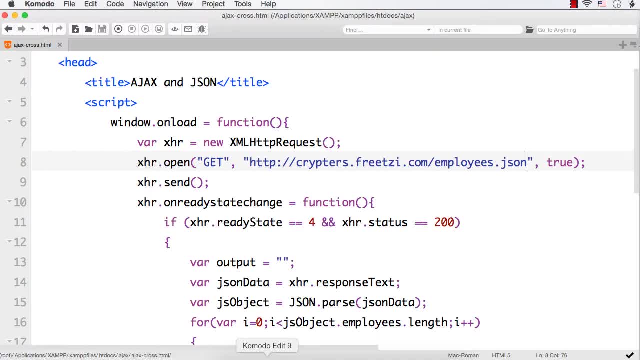 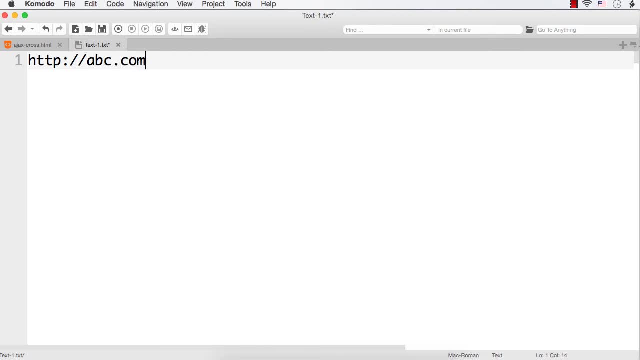 host name and also same port number. so suppose I try to make request from HTTP slash abccom to HTTP slash XYZ calm. this will not be allowed because of same origin policy. similarly, if I try to make request from this HTTP slash abccom to Проаб 있어 equator TPS slash abccom, here also it will not be allowed. 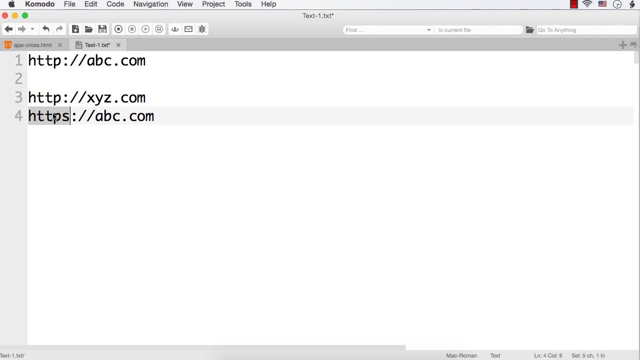 because it is using a different protocol. that is, here it is http//www- denencheesecom- HTTPS and here it is HTTP. and again, if I try to make a request to HTTP slash wwwabccom, Still it will not be allowed because this will be considered as a different domain here.